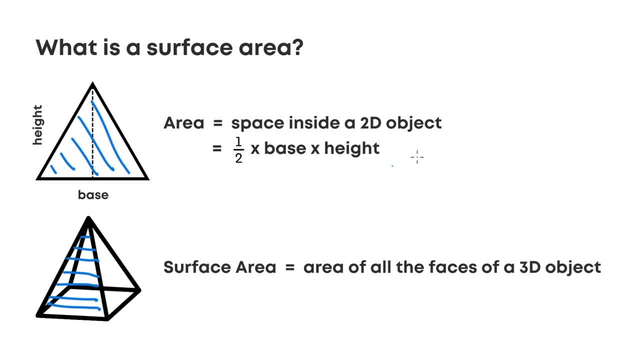 the faces of the pyramid and still calculate the area of that right. But notice how we have all of these surfaces that are on the outside of the pyramid, other faces that we haven't colored yet. So in order to find the total surface area of this pyramid, we need to color all of the faces, meaning we need to. 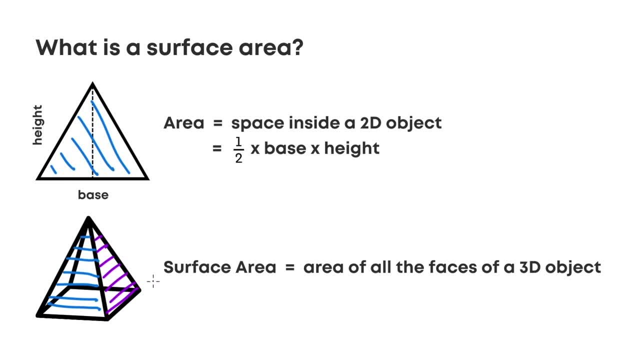 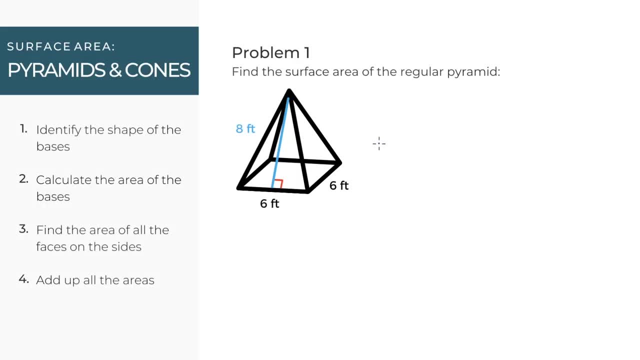 calculate all of the individual areas of the faces and then add it all up. That is the surface area of a pyramid. The most common pyramid problem you'll probably see is one like this, where you're asked to find the surface area of a regular 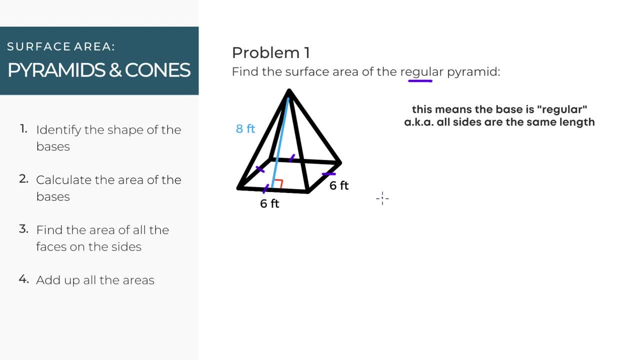 pyramid like this one. In order to solve for the surface area of the pyramid, our first step is just to determine the shape of the base For this pyramid. it looks like this base is a square because there are four sides and all of the 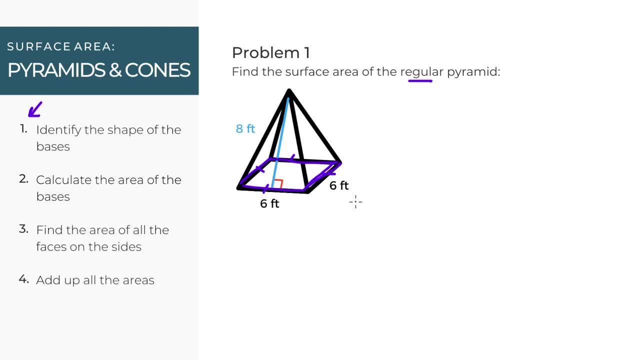 sides are the same length Again, because it's a regular pyramid. Our second step is to calculate the area of the base, and we know, or at least we should know that, that the area of a square is just the base times height. so 6 feet times 6 feet. 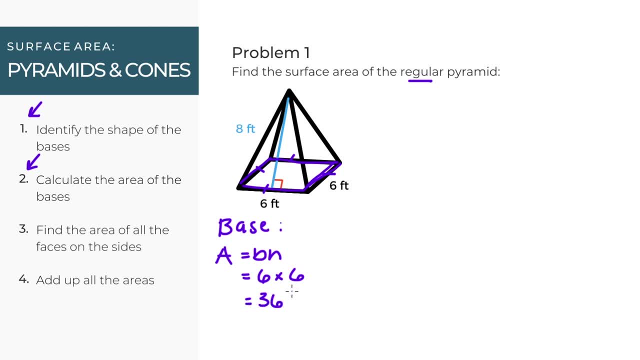 which is 36 feet squared. This is the area of the base. Our third step now is to calculate the area of all the faces. which are these shapes on the sides here? If we look at one of these faces, this is just a triangle right And the area of. 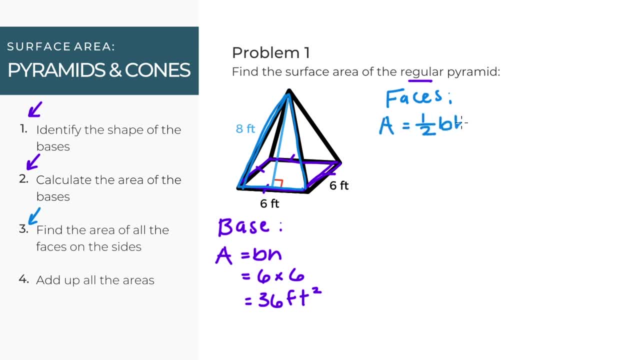 a triangle is 1 half base times height. If I plug in 1 half times the base, which is 6 feet, times the height of the triangle, which is 8 feet, then we get an area of 24 feet squared. Now this is the area of only one of the faces and we 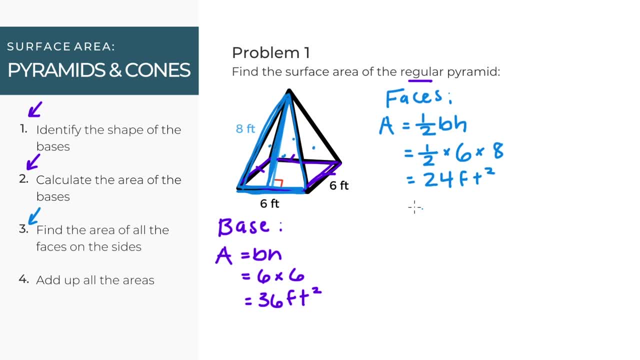 have how many faces- 1,, 2,, 3,, 4 faces- And we need to find the area of all of the faces. so we have to multiply 24 and multiply it by 4, which is how many faces. we have 96 square feet. This is the area of all of our faces on the pyramid. Now 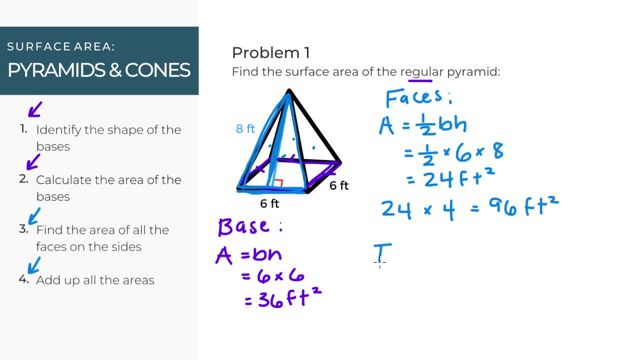 our fourth and final step is to add up all of the areas that we just found. So we're going to add the area of the base, which we found was 36, and then add the area of all the faces, which is 96. And we'll get that, the total surface area of 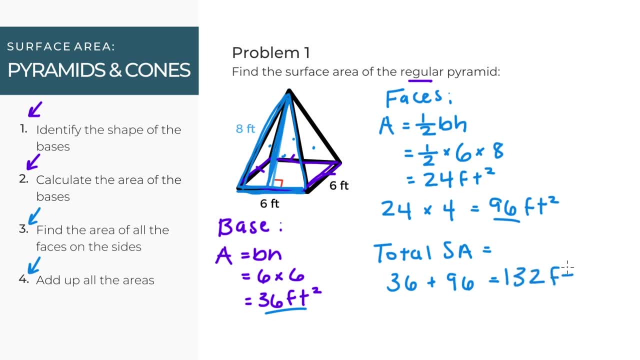 this pyramid is 132 square feet. Just keep in mind this problem might get a little more tricky if this base wasn't regular, meaning not all of the sides are the same length, So maybe this side was 10 feet instead of 6 feet. The steps are: 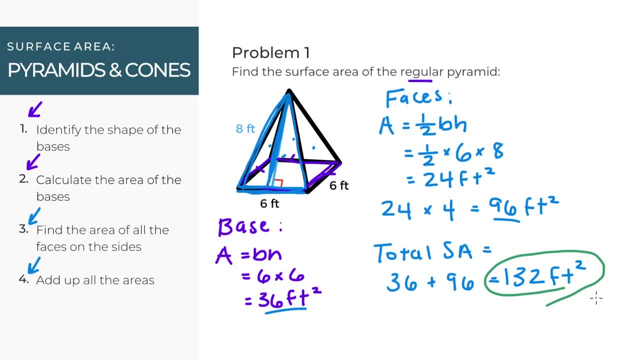 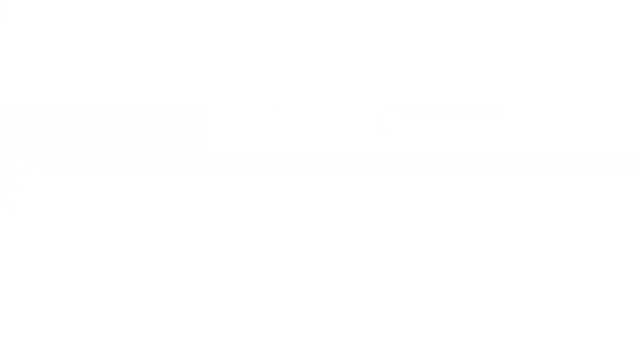 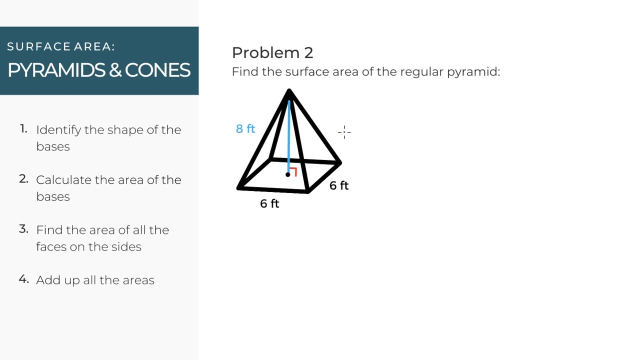 the same, but you can't just multiply the area of the base and the area of the faces by 4 anymore. You'd have to calculate the area of all of the faces separately and then add them up. Alright, problem number 2. Now this problem looks exactly like the problem we just did. 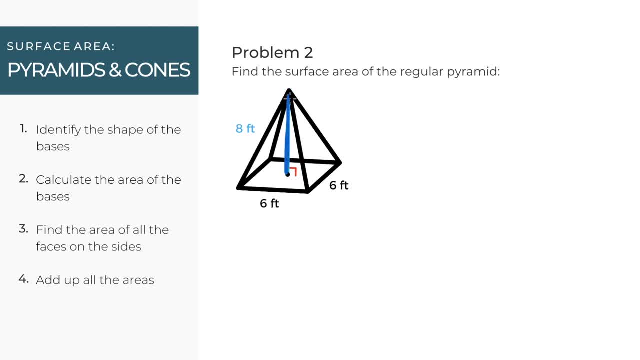 but if you look closely, they're actually giving you the height of the pyramid and not the height of the face of the triangle, And because of that there's a little extra work we have to do. So this is the pyramid, and all of the steps are still the same. Our first step is still: 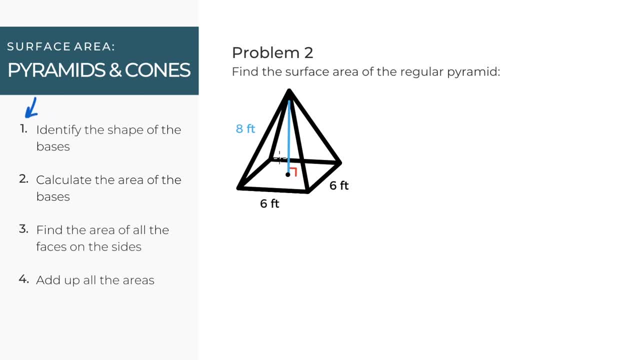 to determine the shape of the base. The base of this pyramid still has 4 sides and they're all still the same length, so the base is a square. For a second step, in order to find the area of the base, we have to find the area of the square, which is calculated by: 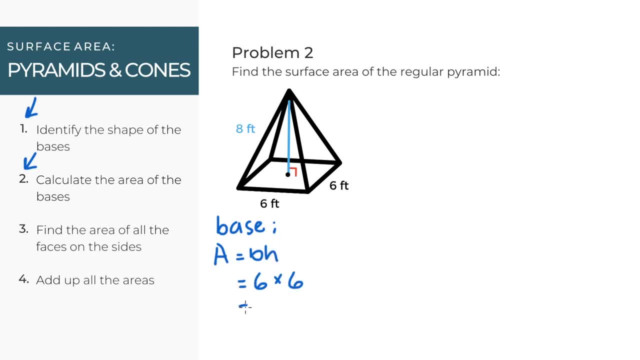 base times height, which is 6 feet times 6 feet, which is still 36 feet squared. Oh yes, sneaky. So far this problem's been exactly like the first one, but for this third step we need to do something a little extra to find the area of the face. 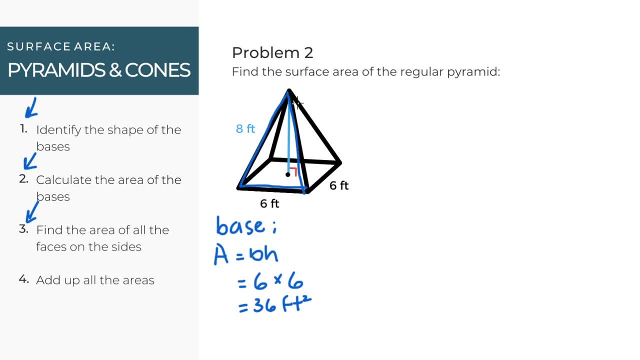 When we look at one face of the pyramid, it's still these triangles here and the areas can still be calculated by using the formula ½ base times height. It was more straightforward back when they directly gave us the height of the triangle, which is this line here: 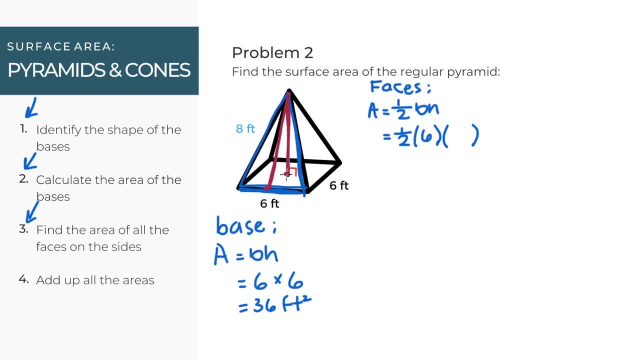 but instead they gave us the height of the pyramid. That was my fault. That was my fault. thing is is that we can use the height of the pyramid to calculate the height of the triangle. If you imagine drawing a line connecting these two heights, this: 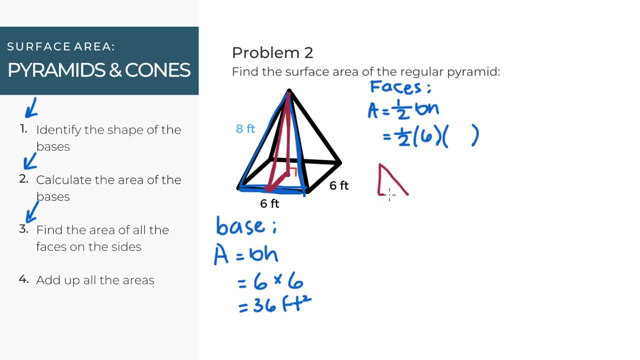 will actually become a right triangle And if you remember, back to the Pythagorean theorem, there is a formula that relates the lengths of these three lines together in a right triangle, which is exactly what we need. The Pythagorean theorem is: a squared plus B squared equals C squared. We already have A, which 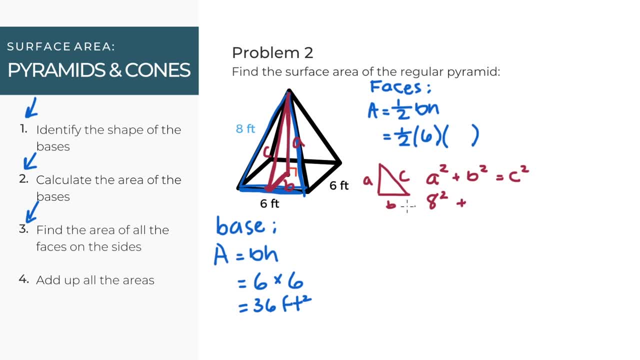 is 8.. We can calculate b, because this length is just half of the length of the side of our square, So one-half of 6 feet, which is 3 feet, And now all we're missing is C. This equation simplifies to: 64 plus 9 equals c squared, and solving 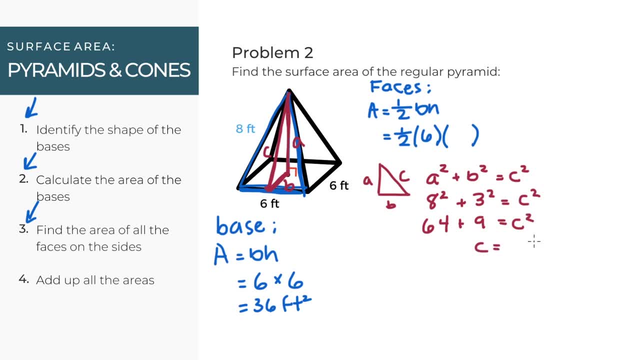 for c. we get that. the height of this triangle is the square root of 73 feet squared. Not the prettiest number, but that is the height of our triangle, And by now I've sometimes forgotten what we're even solving for. but if you remember, we're still on that third step. We're trying to solve for the. 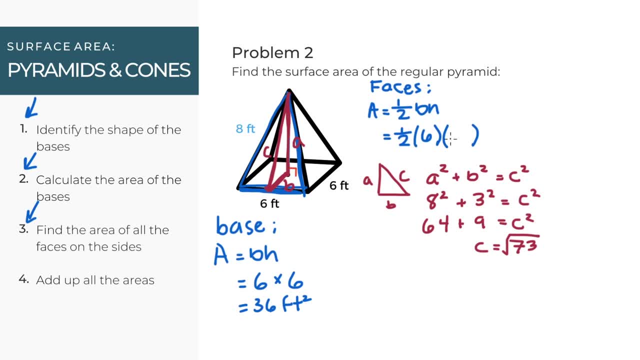 area of the faces, which is this triangle. We can finally use the formula for the area of a triangle, which is one half base times height, because we actually know the height of our triangle now. So, plugging in six for the base and the square root of 73 for the height, we get that the area. 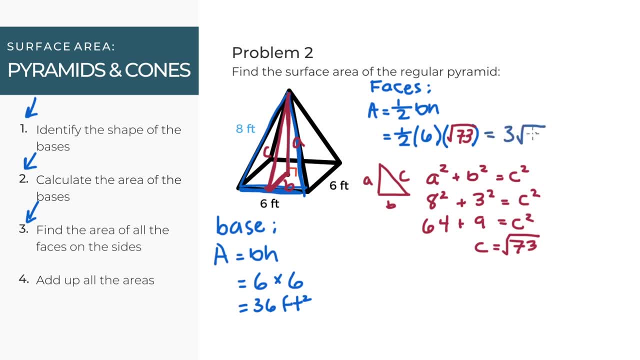 of one face is three times the square root of 73.. Now remember that we have to find the area of all of the faces right, and there are four faces on this particular pyramid. We know that this is a regular pyramid, so all of the faces are the same and they have the same area. 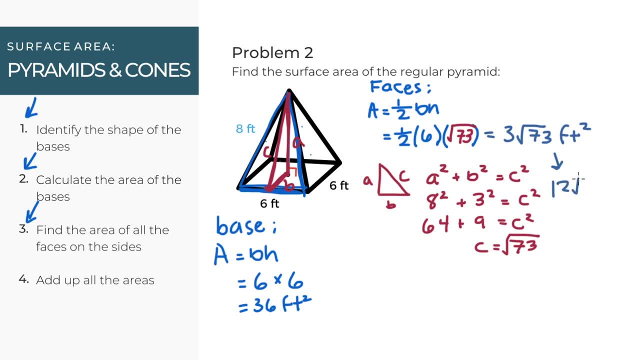 so let's multiply this area by four and we'll get 12 times the square root of 73.. This is the area of all of our faces added together. Now we are at step four, which is to add it all together, the area of our base plus the area of 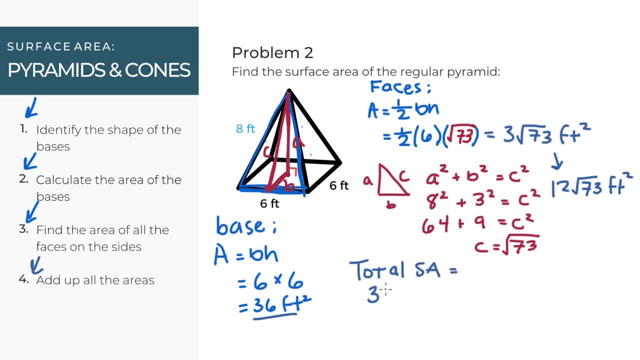 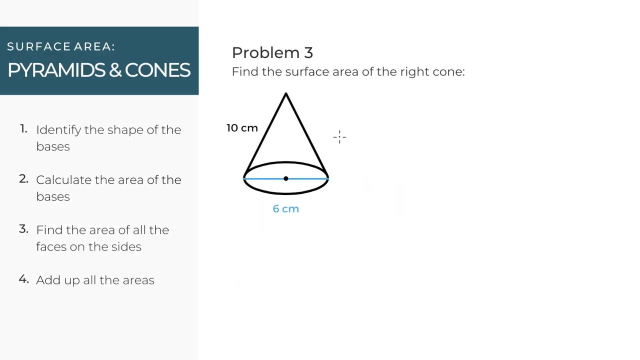 all of our faces. So 36 plus 12 times the square root of 73, which is roughly 138.5 square feet. This is the surface area of our pyramid. Let's now try for the surface area of a cone. Even though the shape is a little different, again, the steps to get the surface area are the same. 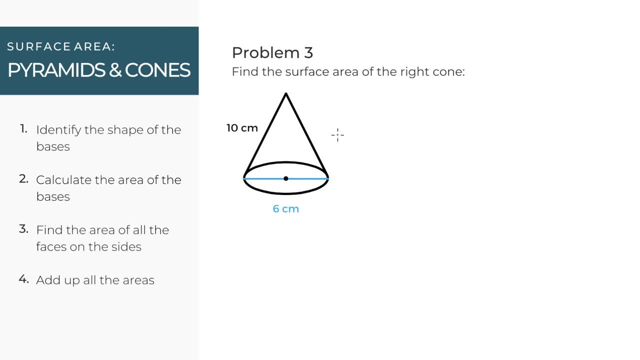 Our first step is to identify the shape of the base and, if you think about it, a cone is pretty much the same thing as a pyramid, except the base is a circle. For our second step, we need to find the area of the base which is a circle. 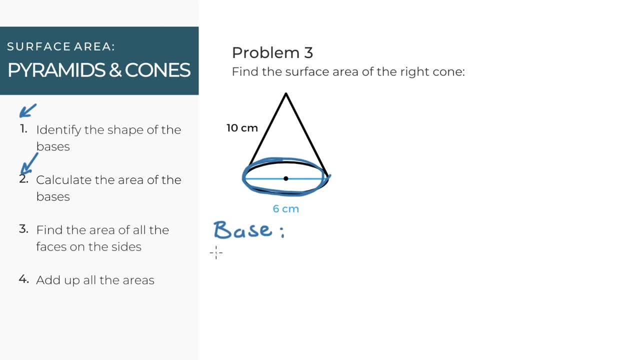 You can find the area of a circle by taking pi r squared, where r is the radius of the circle. You'll notice that this circle has multiple bases, but on the surface it's only one base and the base is one circle. You'll notice that the diagram says that the diameter of the circle is 6 cm, so the radius. 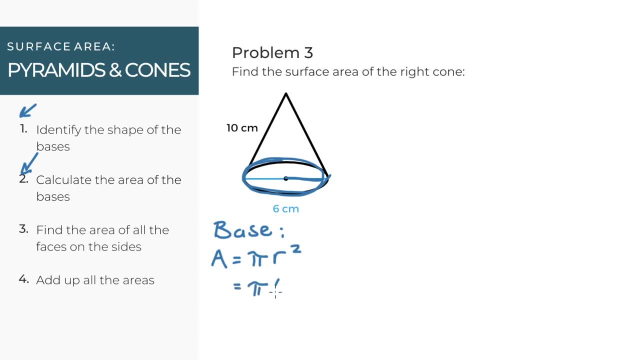 is one half of that, which is 3 cm. Pi times 3 squared is about 28.3 cm squared. That is the area of our base For our third step. we need to find the area of all of our faces which is actually the. 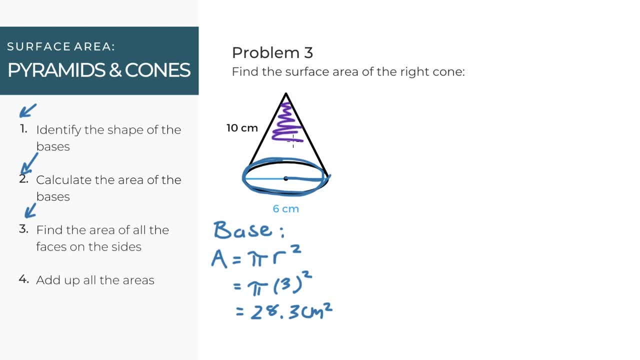 smooth surface all around up here. Now I want you to imagine that you have a paper cone and if you cut along the edge here and unravel the paper, you'll actually get something that looks like a slice of pizza. This is actually the face of our cone. 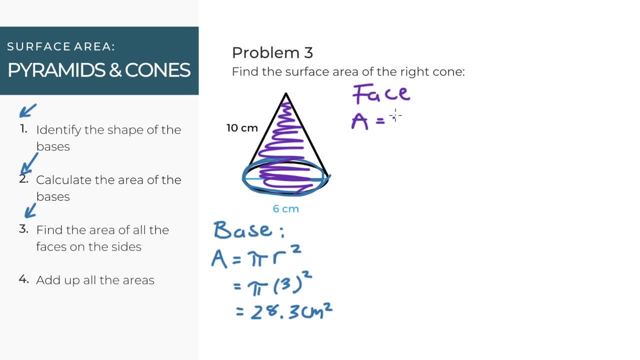 And this is where you kind of just have to remember that the area of this pizza slice is equal to pi r s, where r is the radius, s is the height of the cone But the slant. here Sometimes you'll see s written as l, but in this case we're writing it as s. 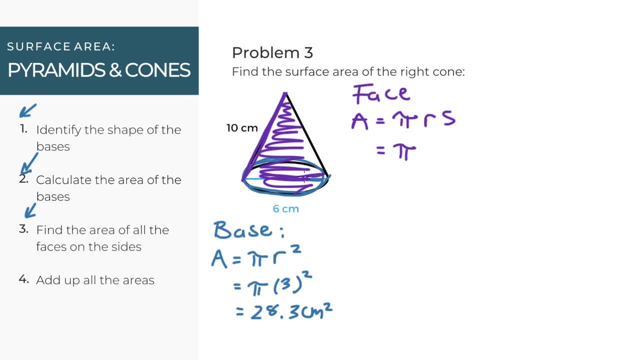 If you plug in, we have 5 times the radius, which we figured out earlier was 3, times the slant height, which is 10.. And this all equals to about 94.2 cm squared. Our last step is to add all of the areas up. 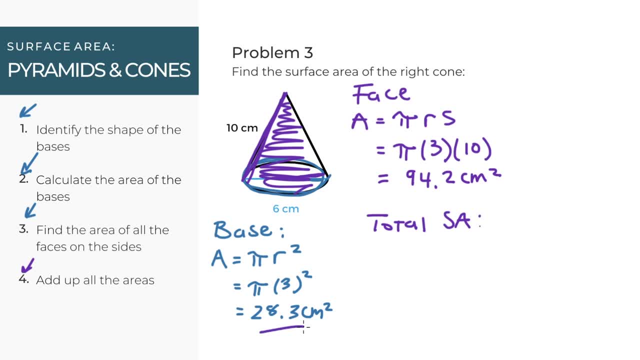 The area of our base was 28.3, and the area of our face or our pizza slice was 94.2.. Adding them up we'll get 122.5 cm squared. This is the surface area of our cone. Similar to our second pyramid problem, we might get a cone problem. that looks initially. 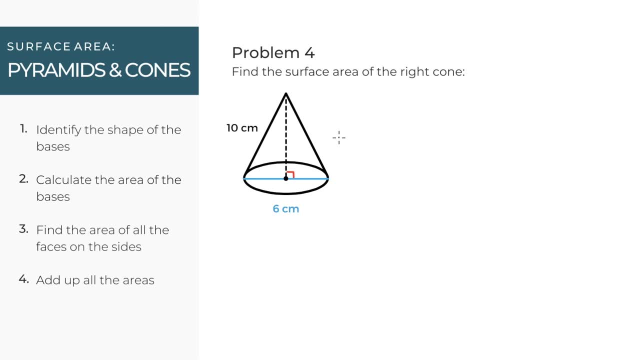 exactly like the same as our last one, but you'll notice that, unfortunately, they gave us the height of the cone, which is not necessarily the same as the slant height we were talking about earlier. So don't fall into the trap: These heights are not the same. 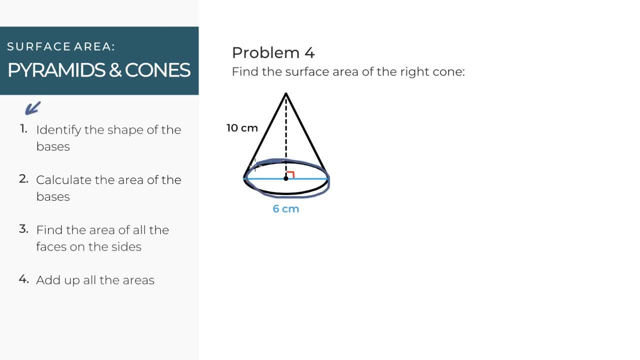 But let's approach the problem in the same way though. Step 1, the base is a circle. Step 2, the area of the base or the circle, is pi? r squared. Our radius is 3 feet, So our area is roughly 28.3 cm squared. 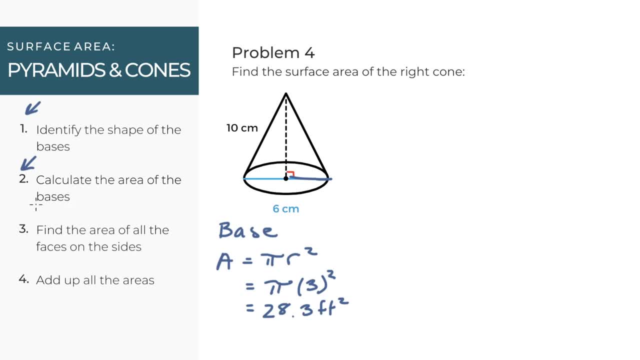 Step 3, we need to find the area of the faces, or face. If you unravel the cone, it becomes our pizza slice again, And the area can be calculated by pi r, s, where r is the radius and s is the slant height. 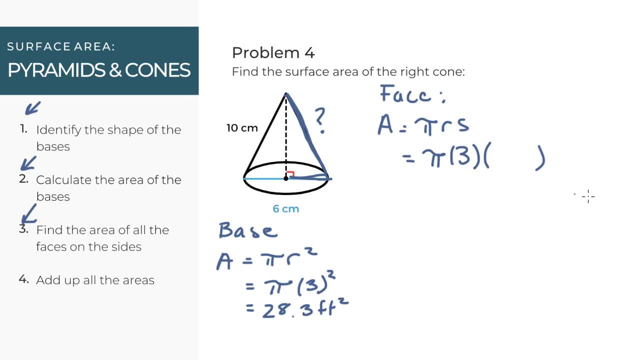 which is this line here. This is where the extra work comes in, because we're not given the slant height. Instead we're given this one, which is just the height of the cone, Kind of like what we did for problem number 2,. we can draw a right triangle connecting. 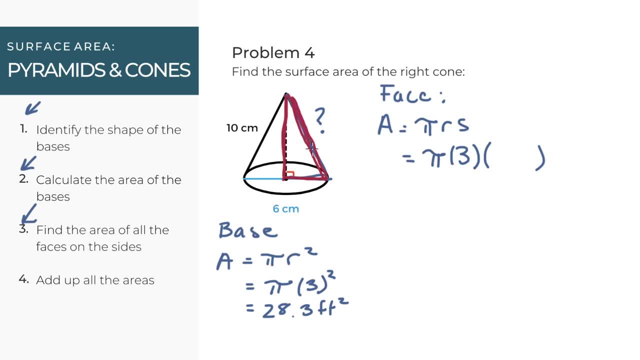 the two lines like this and then use the Pythagorean theorem. The Pythagorean theorem relates the lengths of the sides of a right triangle And it is: a squared plus b squared equals c squared, Our a, we know, which is 10.3 cm squared. 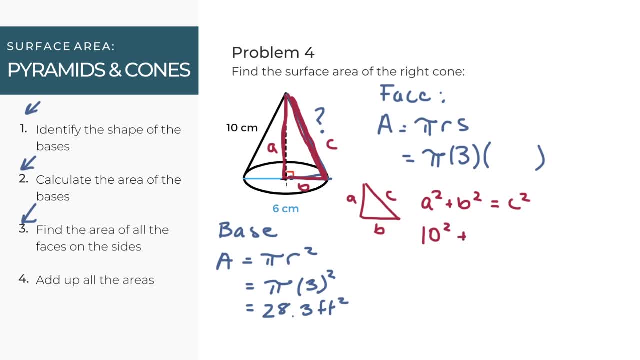 So we're going to use the Pythagorean theorem, Step 2, we need to find the area of the base. We have a square root of 10 cm, b is half of 6, which is 3.. And we're trying to find c.